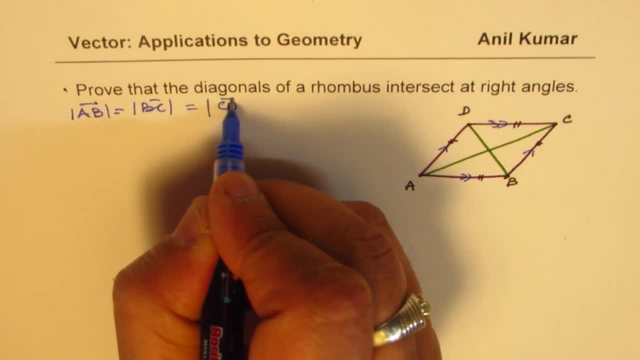 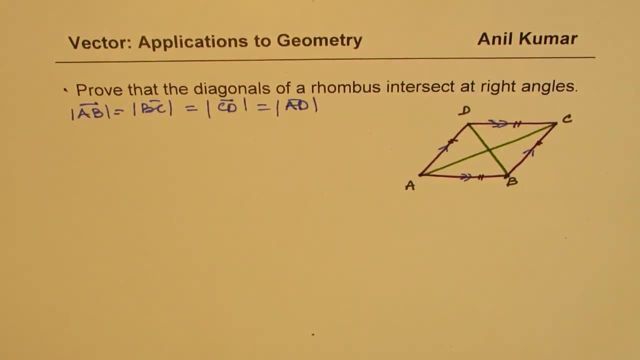 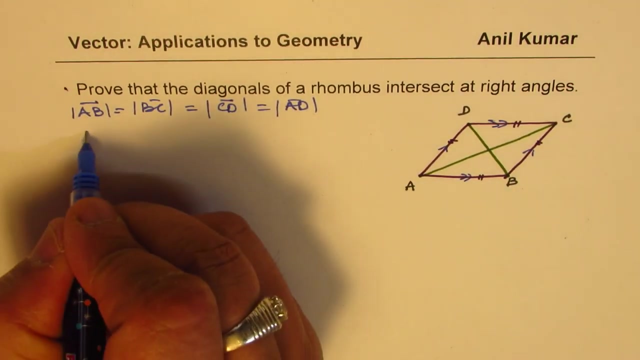 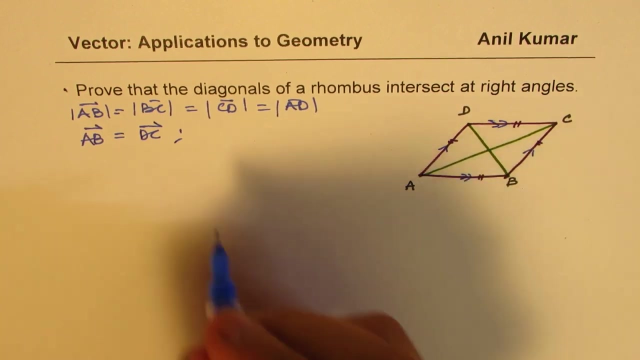 which is equal to the magnitude of CD, is equal to the magnitude of AD or DA, right? So that is given to us and we are also given that they are equal vectors. So AB vector AB is actually equal to vector DC and the vector AD is equal to vector BC, since it is a rhombus. 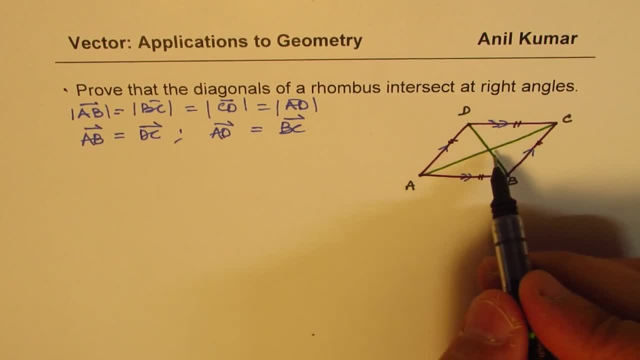 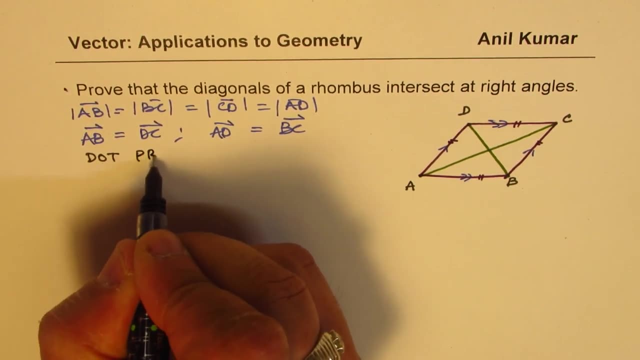 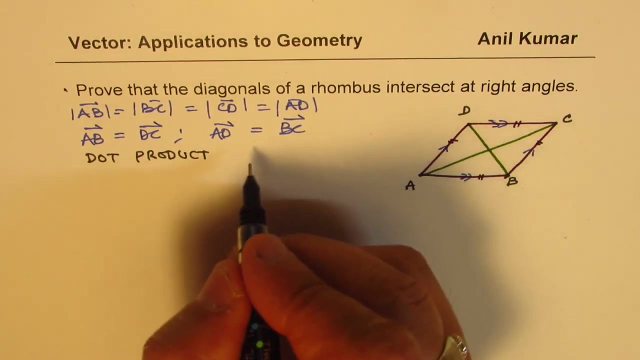 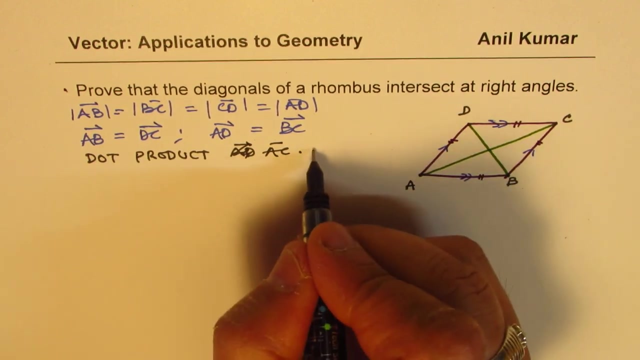 ok, Now to prove that they are intersecting at right angles, we will find the dot product right. So, basically, the concept is that the dot product of these two diagonals, which is AB and BD, AC, and sorry, AC and BD, should be equal to 0, right? so that is what we want to. 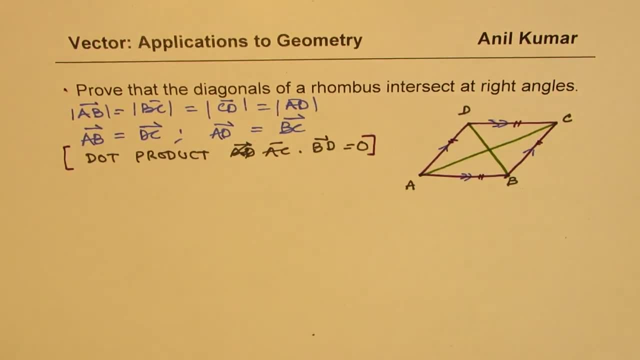 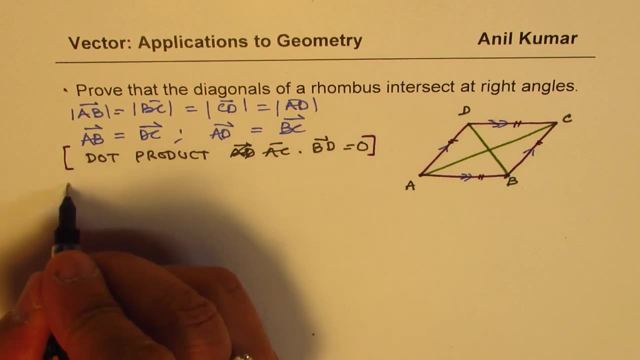 prove. basically, if that happens, then they are intersecting at right angles. okay, so let's begin by finding what the dot product is. so let's see what is dot product of AC with B to D. now AC could be written as a combination of a, B and. 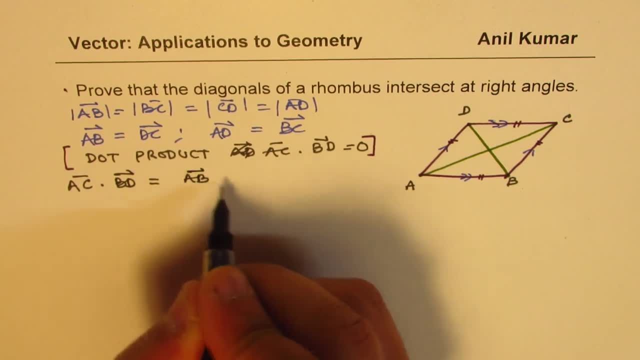 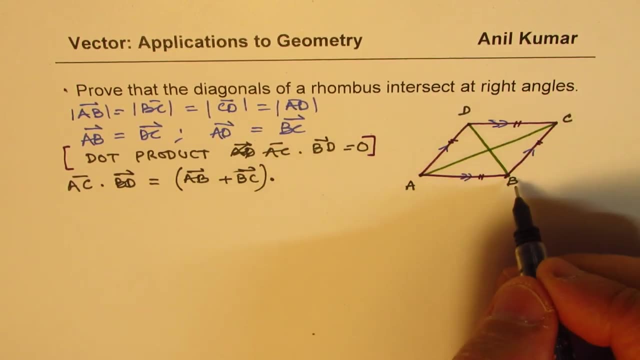 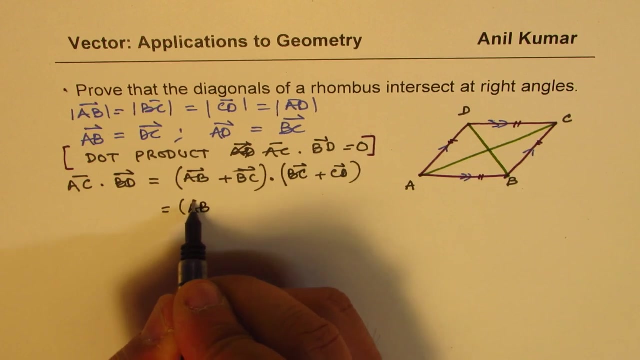 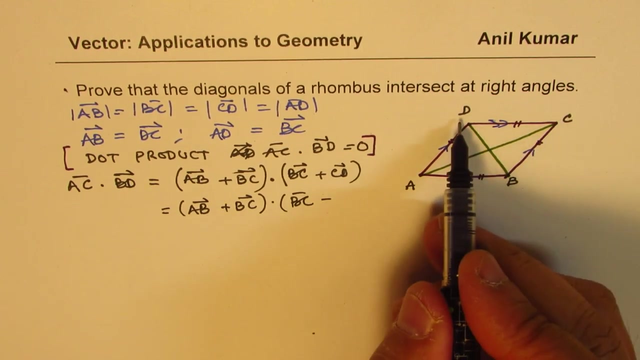 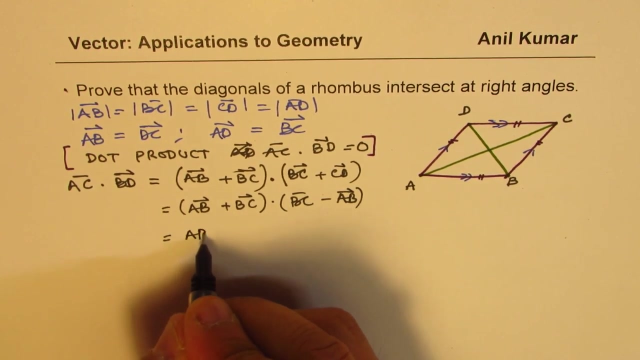 BC. so we could write this as a B plus BC, dot B to D is CB, BC plus CD, correct? so now AB and CD are opposite vectors. so I could also write this as a B plus BC, dot, BC minus instead of CD with rate AB. right now let's expand so we have a B dot BC and then we have minus sign a B.